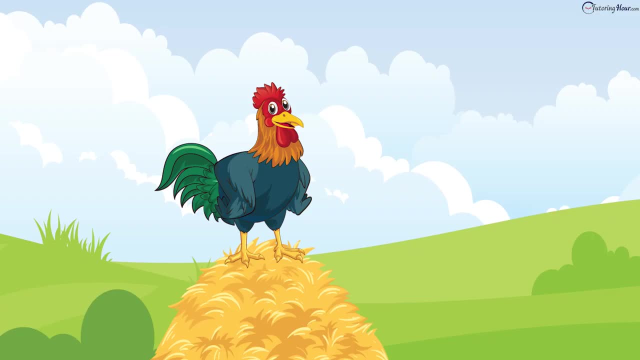 Telling Time to the Hour. Hey, I'm Doodle, the rooster who wakes you from your sleep every morning. I love telling the time, and today I'll show you how you could be as good a time teller as I am. 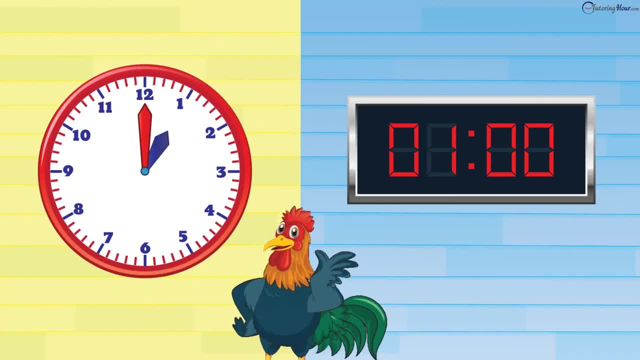 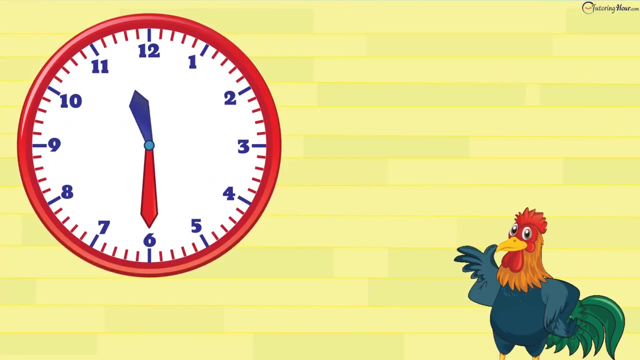 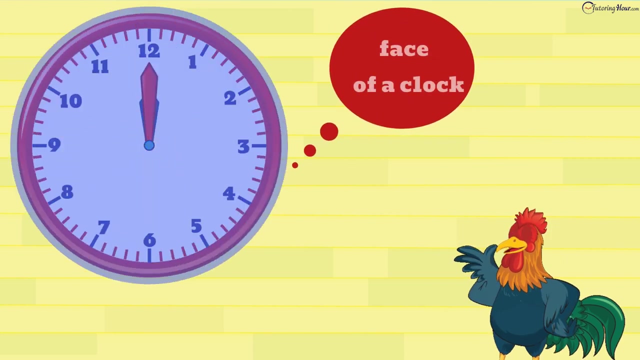 First things first. there are the two types of clocks. This is an analog clock and this is a digital clock. Digital Clock: Reading a digital clock is very simple, but reading an analog clock can be a little tricky. Let's take a look at the analog clock. This whole thing is called the face of a clock. 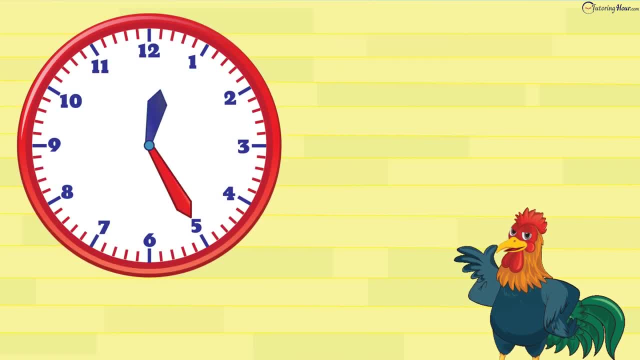 It has two hands: a short hand and a long hand. The short hand tells what hour it is and it is called the hour hand. The long hand is called the minute hand. An analog clock is marked with numbers 1 through 12.. 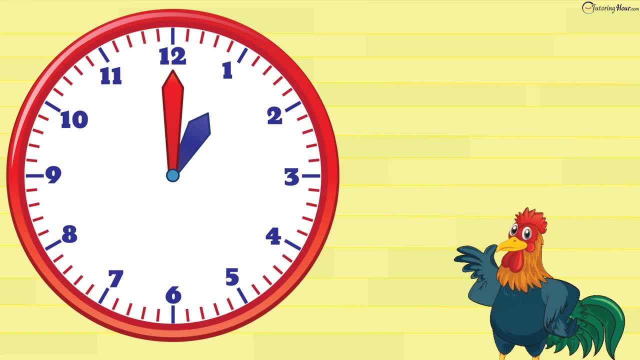 Let's take a closer look at our clock face. The hour hand is pointing to 1, and the minute hand is pointing to 12.. When the minute hand is pointing to 12, you need to say o'clock, So we say it is one o'clock. 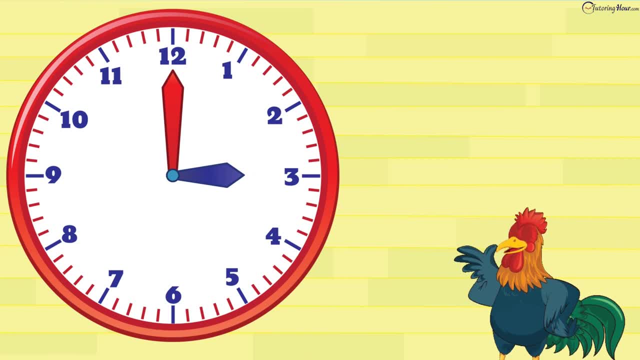 Look at the clock now. Where is the hour hand? It is at 3, and the minute hand is at 12.. So what time is it? It is 3 o'clock. Look at the clock now. What time is it? 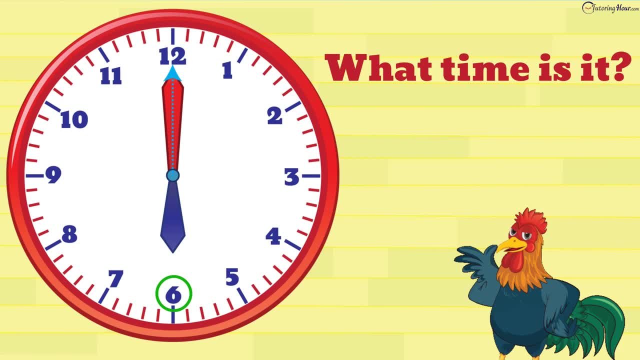 The hour hand is pointing to 6, and the minute hand is at 12.. So it is 6 o'clock. Look at the clock now. What time is it? It is 9 o'clock. Look at the clock now. What time is it? Both the hands are pointing to 12, which means it is 12 o'clock. 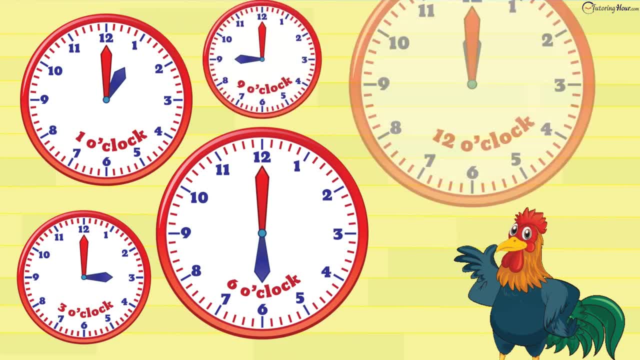 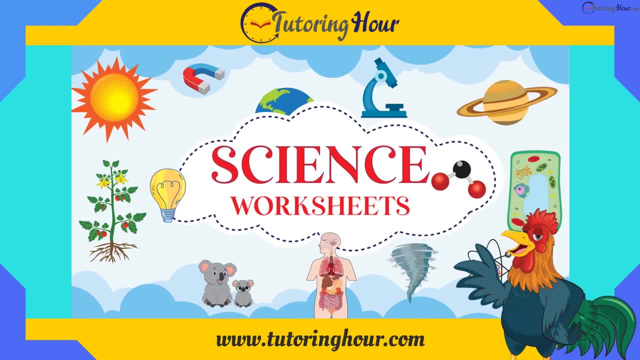 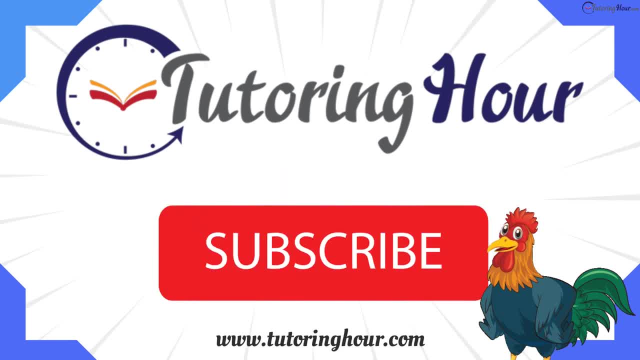 I'll go get some sleep Like and subscribe to Tutoring Hour and stay tuned for regular updates. Bye-bye.